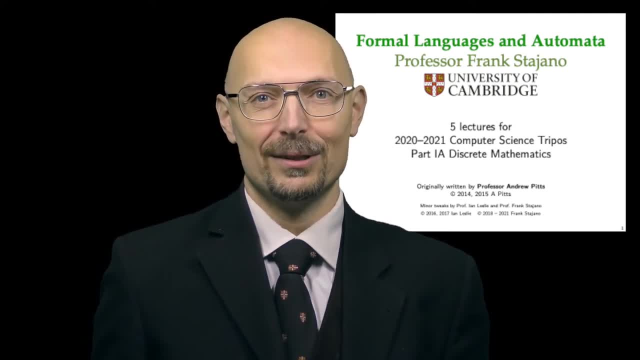 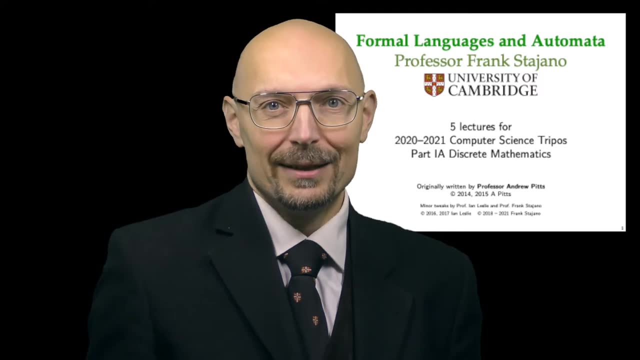 Welcome to Frank's Diana Explains and to the formal languages part of the Discrete Mathematics course at Cambridge. Even though this is a first-year course, by the time I get here, a fair number of you has already been exposed to regular expressions, perhaps through Unix tools. 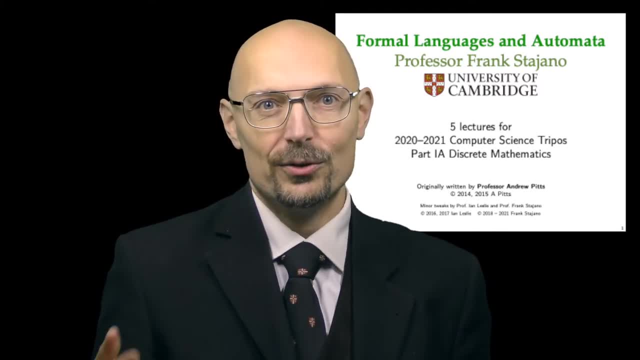 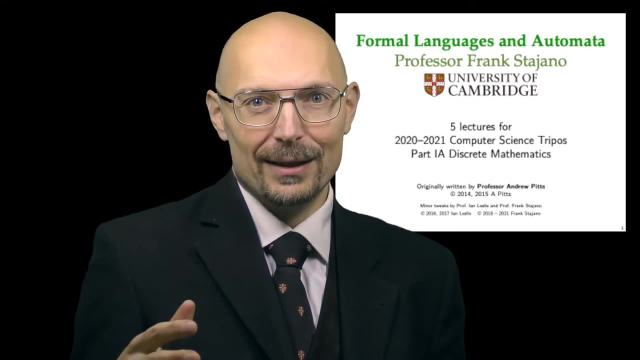 such as grep or Emacs, or maybe because you've used regular expressions in a scripting language such as Python or Perl. In this course, I'm not going to teach you how to write and debug complicated regular expressions. We shall instead concentrate on the fundamentals. 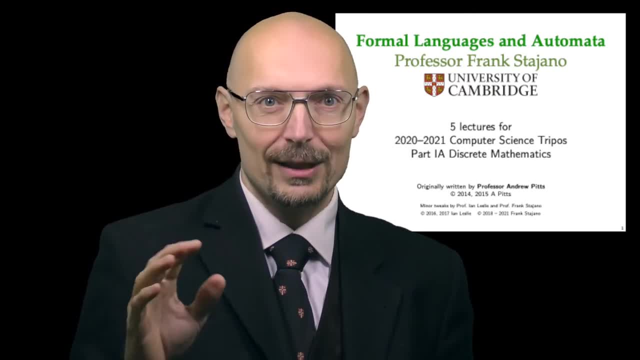 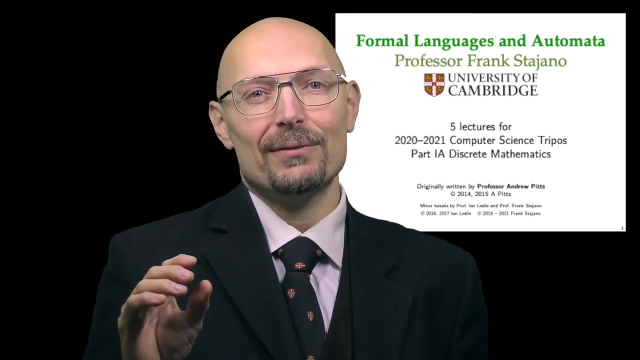 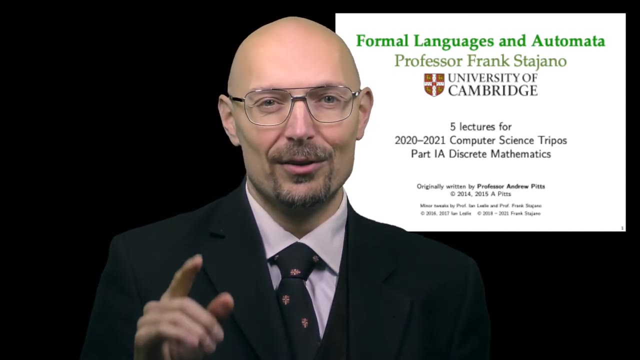 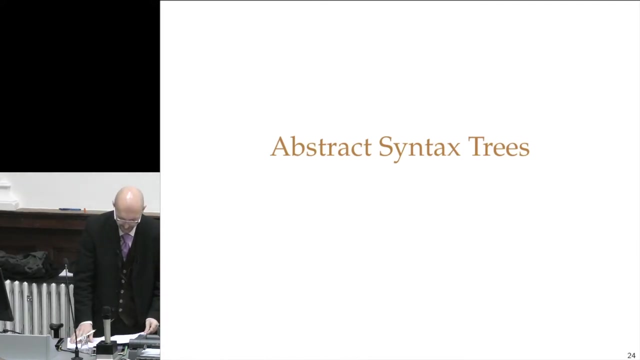 on the expressive power of regular expressions, on their limits and on how they relate to regular languages, And we shall start with a very mathematically flavoured distinction between concrete and abstract syntax that you probably never saw when you encountered regular expressions before. So the next section of our deck of slides talks of abstract. 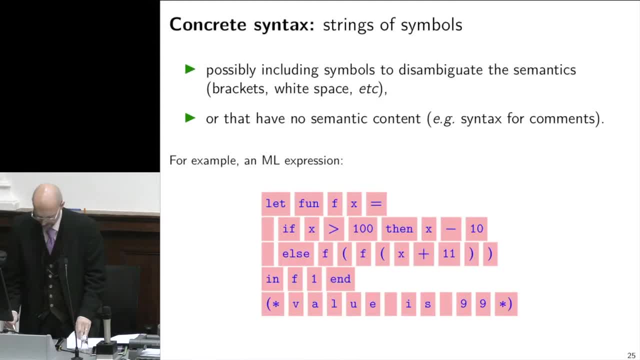 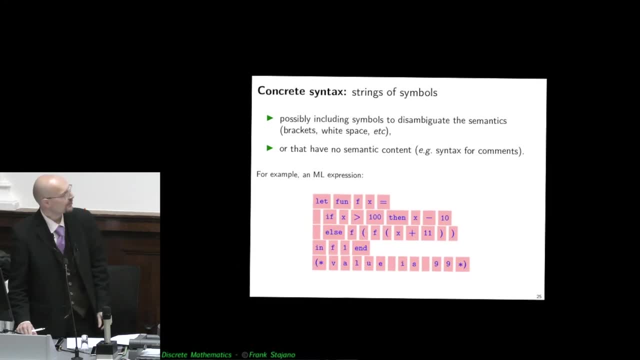 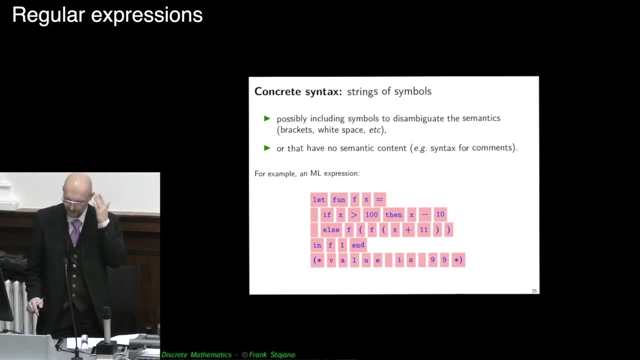 syntax trees: Abstract syntax trees, and then the next slide instead says concrete syntax. So are we talking abstract or concrete? Well, the concrete syntax is a set of symbols and the abstract syntax is a way of representing things in the concrete syntax, in a slightly more general way. And if I'm just going on like this, then things make little sense. 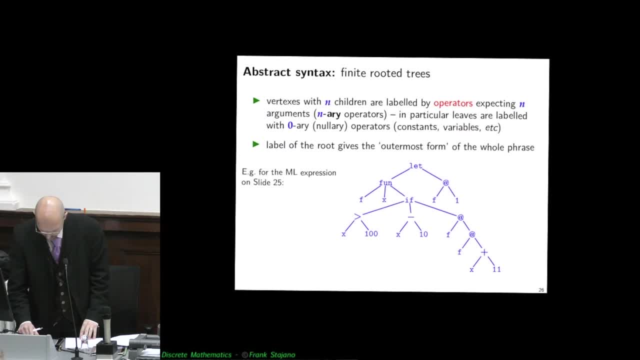 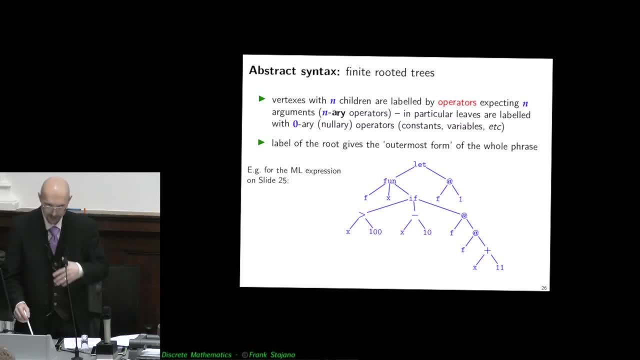 So I'll just show the abstract version of what we had previously, where these are things that are not linearised into a sequence of symbols. They're represented here as a tree, And the nodes in this tree are vertices which combine subtrees, And so the let is a thing that combines this function over here. 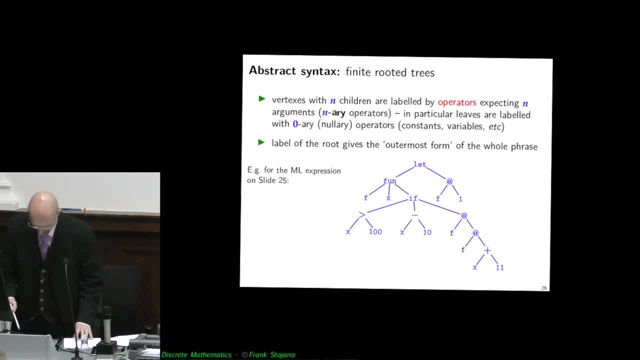 which is started by this fun. In fact, I should really be taking the previous slide again. it's a bit of a pain to do it. I'm relating sub-expressions of my previously linearised concrete syntax into chunks that make sense according to what the meaning of this is, But at the moment 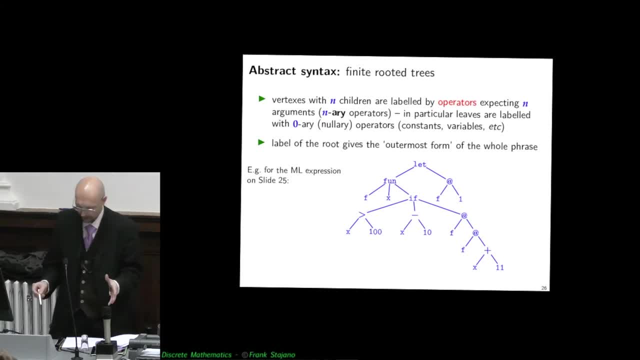 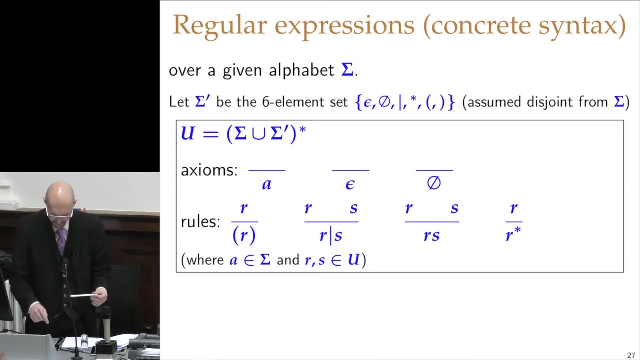 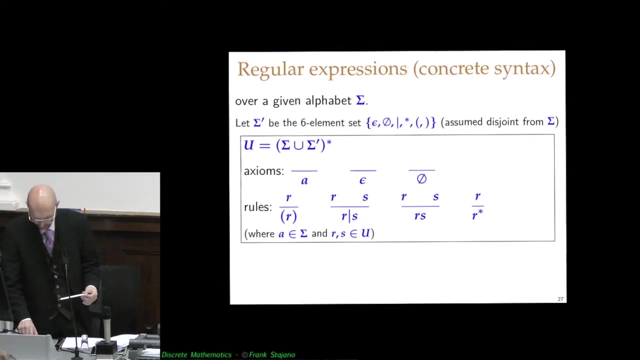 I'm not really interested in the meaning. I'm interested in their structure, And this gives me some structure which the concrete syntax doesn't quite show. We are making this introduction because we want to give syntax for regular expressions. Regular expressions is something that this is supposed to teach you from zero. 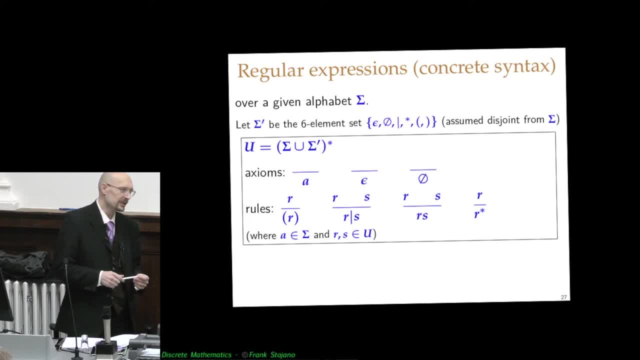 but every time I get to this point I see people have already seen regular expressions to death. Is there anybody in the audience who has never worked with regular expressions? Then hands up if you've never seen regular expressions. There's two, three, four, five, six, Ah, coming out of the woodwork. 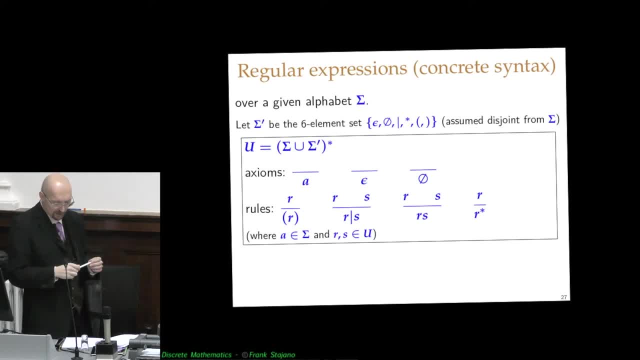 now, Okay, right, There are a few people who've never seen regular expressions. Okay, for their benefit. regular expressions are a way of expressing patterns in the spirit of when you are in the command line shell and you say, instead of naming files, you say list all the files that finish. 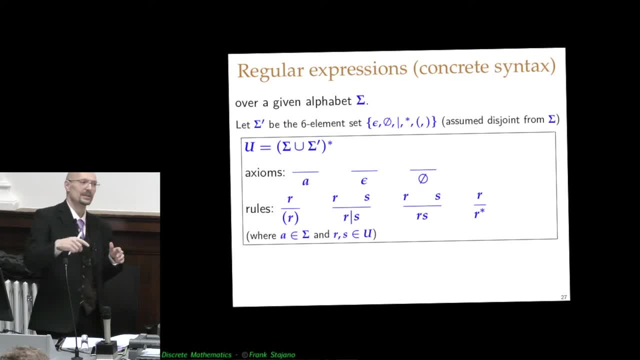 with dot txt by putting star dot txt. That's a way of expressing a pattern. That pattern is not a regular expression. The regular expressions are a mechanism for expressing more complicated patterns and there also exists an asterisk in there, but it has a different meaning. It doesn't mean replace. 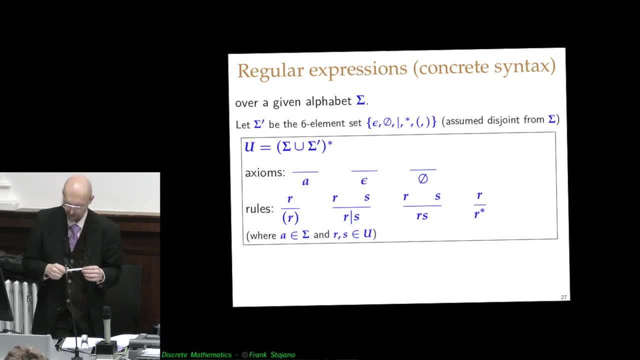 with any character. It means repeat the previous regular expression zero or more times And, in fact, the regular expressions as we are going to define them in this course, which are a kind of strict, no-frills version of the regular expressions that you might find in your Unix tools. 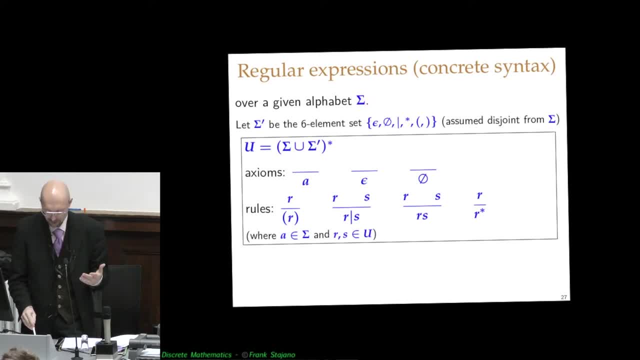 are based on the alphabet of the strings, plus these meta symbols that don't occur in the actual strings of your language. And these symbols are this other epsilon. and notice the difference between this shape of epsilon and the other one that we used previously, which looked like this: It's not the same as this epsilon. 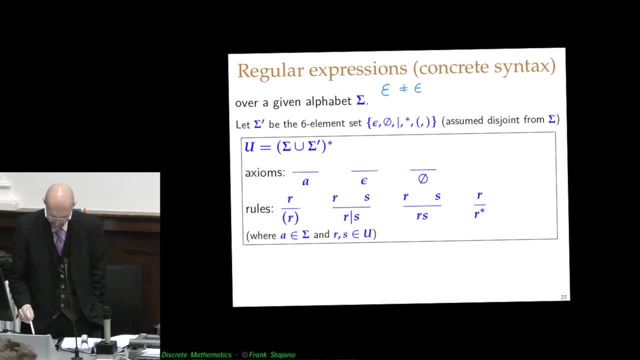 So this epsilon over here meant the empty string and this one means a regular expression matching the empty string. This symbol that looks like the empty set means a regular expression that never matches anything. This vertical bar means the alternation of two things. 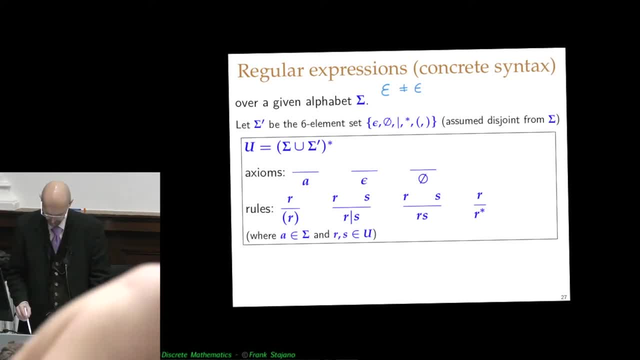 so you can take the thing on the left or on the right. This asterisk means repeat zero more times and these brackets are there to express precedence. So the regular expressions are sets of strings over the alphabet given by the alphabet of your basic strings and the meta symbols. 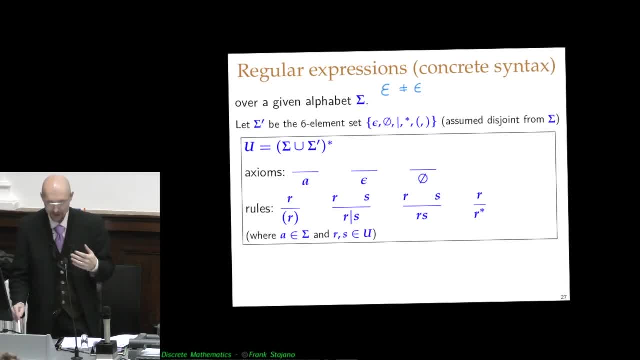 Regular expressions in concrete syntax are themselves just strings of these symbols, and I'm going to inductively define the shape of a syntactically correct regular expression by saying that any of the symbols in sigma is a valid regular expression, this special epsilon that says a regular expression. 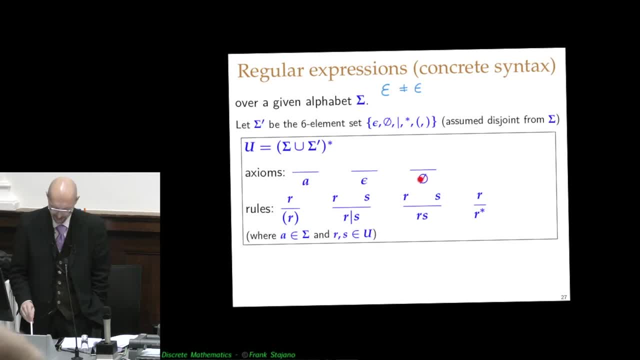 matching only the empty string is a regular expression. this other meta symbol which means regular expression, matching nothing else, is also a valid regular expression. and then if the things on top are regular expressions, then the things at the bottom are also regular expression. wrapping one in brackets, alternating between two of them. 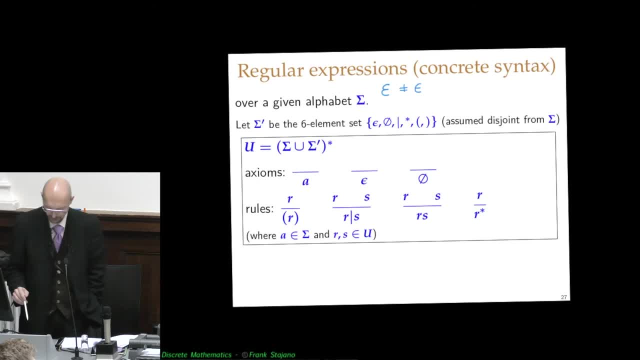 concatenating two of them and repeating one of them zero or more times, and I'm actually cheating because I'm telling you what they do as opposed to reading out the concrete syntax. at this stage, we are strictly only speaking about what they look like on the piece of paper. we are not saying anywhere what the 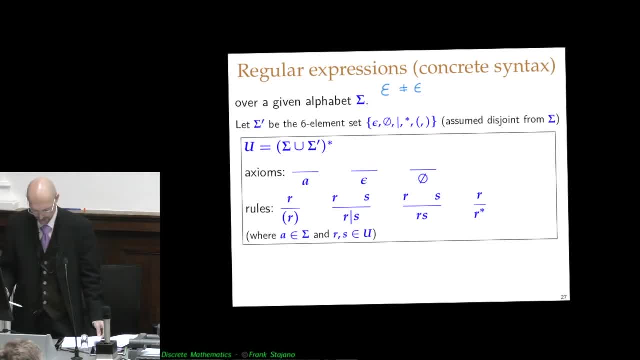 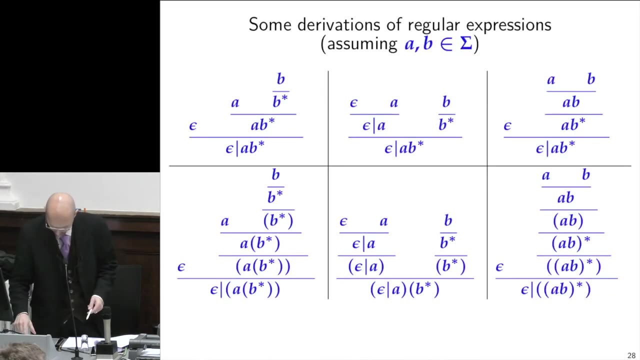 semantics would be, whereas I'm talking about the semantics because I assume that you are, I assume most of you are familiar with regular expression. for those who are not, we should have an example, and I hope the slides have an example, though I don't know the slides by heart. this is not an example of 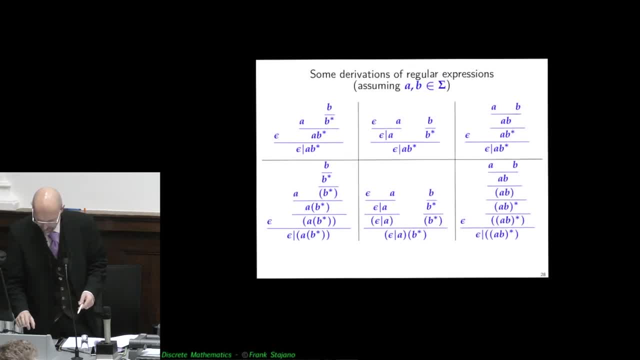 regular expression is just an example of deriving syntactically correct regular expressions from the inductive rules that we just had. and this is just six derivations for various regular expressions which you can work through and you see that they match. now the interesting thing is that in this row, 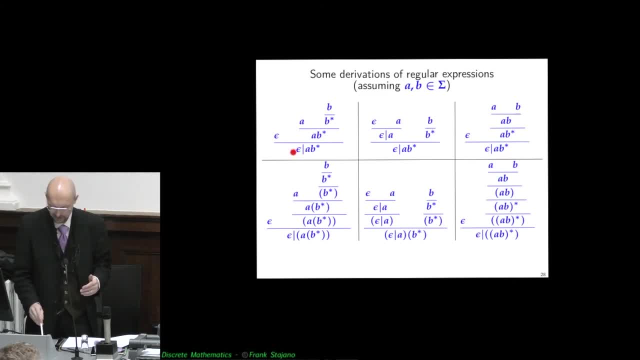 over here. these three derivations lead to this regular expression, which is triply valid as a syntactic correct regular expression. but if you, if your brain is still switched on and you're not just thinking right, there's only five minutes before he closes and I can finally go to lunch. if you're instead 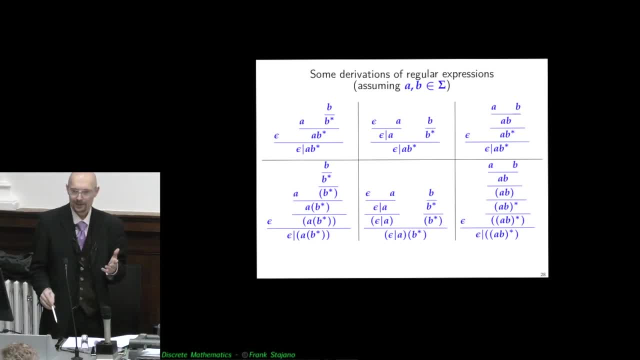 still thinking about this. you should be quite upset. how many of you are upset? well, a small minority. okay, we'll have lunch soon for all the others, don't worry. so you're upset because you're saying, well, only one of these really makes sense. the other things is like they're violating the priority that we should be. 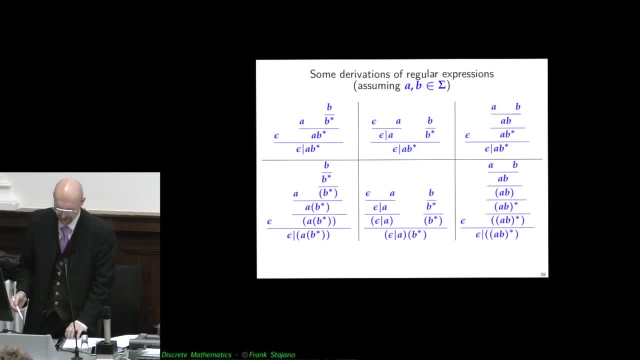 having over these operators, and you would be correct in saying that. but actually we are just doing formal stuff, mathematical stuff, where the only things that work are the things that we have said. so if we haven't said there is precedence, then there isn't yet, but at some point we'll say it, and so there. 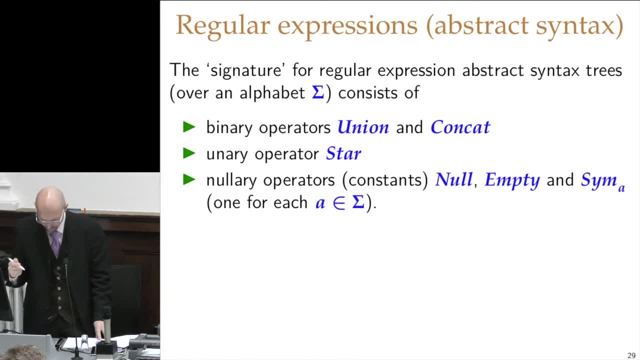 will be, but until then, there is it. so this is now the move between the concrete syntax, which is the strings of symbols and mechanisms- symbols, we have seen, which can be combined in the ways prescribed by the inductive rules- and the abstract syntax. the abstract syntax is the way that you 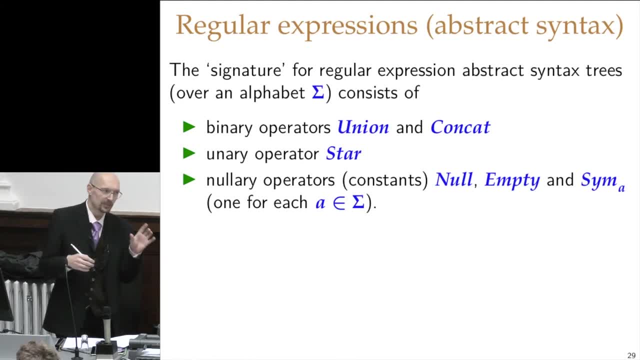 would have the regular expression inside your computer when you're going to operate on it, and it's something that respects its structure, and so you map each of the regular expression operators to one of these primitives here: binary operators, union and concat. unary operator, star. nullary operators, null. 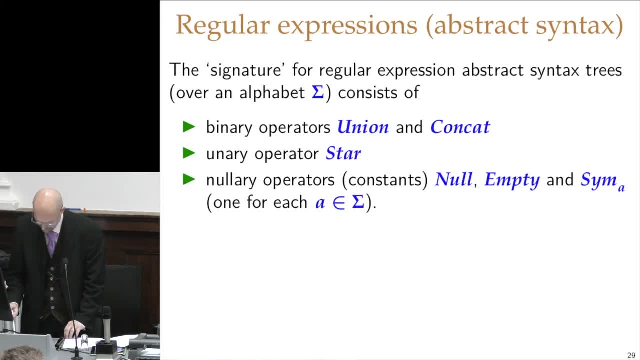 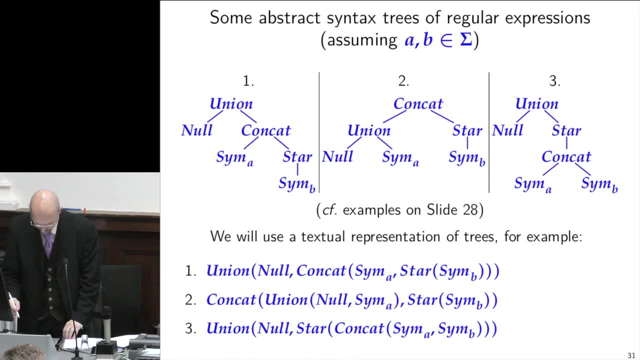 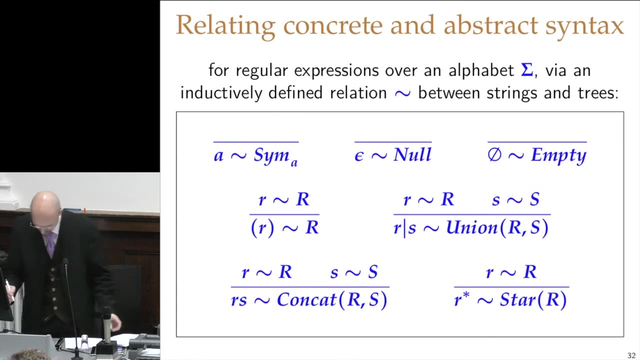 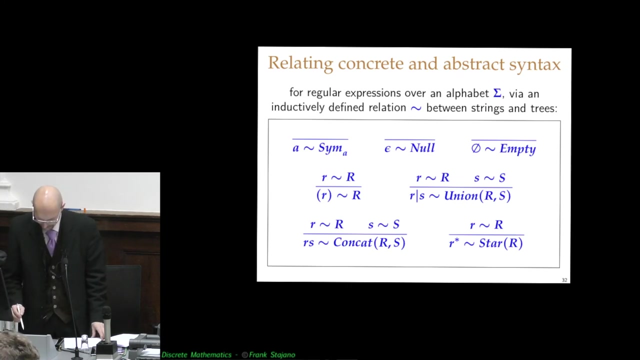 empty and symbol a, one for each a, and notice this is same thing expressed in the OCaml syntax. notice here, or maybe here we are on slide 32 now. notice that, um, there is something mapped to something that didn't even have a symbol in the regular expression syntax. so when we express the syntax we have, we have these: 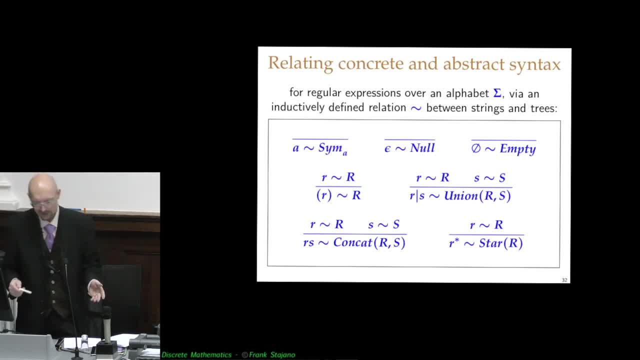 symbols: the funny epsilon, the funny empty set, the brackets and blah blah, and we didn't have any symbol for expressing the concatenation. so it's not like I'm getting one of those abstract syntax operators for everyone of the meta symbols. no, the concatenation is something I do by just putting things. 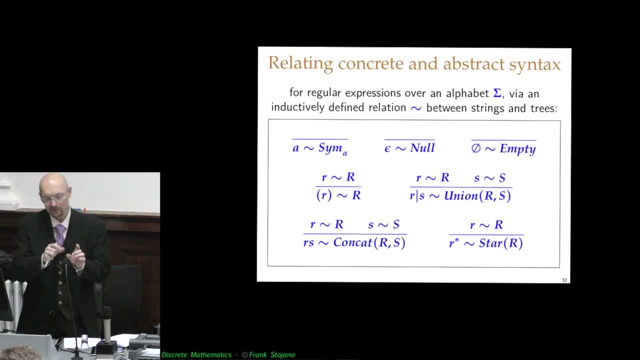 together. so it doesn't have any special symbol in the concrete syntax of regular expressions, but it corresponds to a major manipulation, which I represent as concatenating this original regular expression and this other one. so the stuff that you see here is this is the mapping between the concrete syntax and 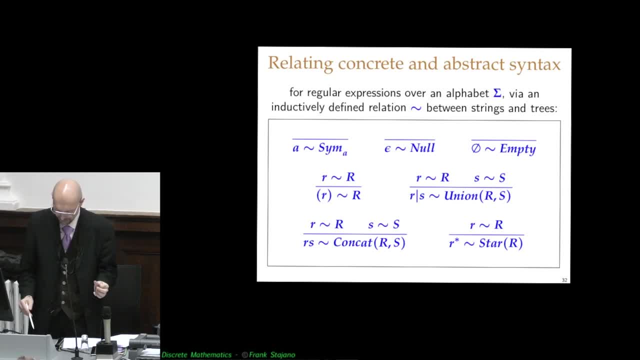 the abstract syntax and in in the case of the Union you have this. so syntactically it looks like just another identifier, but here you have an operator in the concrete syntax, here you don't, and here you have an operator instead, in both cases in the. but still it doesn't matter which group. what method should I use? 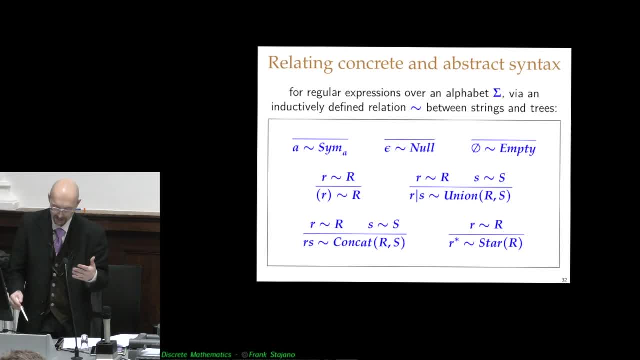 abstract syntax, and yet at no point here have I said what the actual semantics would be in the case of union. it means if my string matches either this or this, then it will match the combined regular expression, and in this other case if the first part, if the string can be split into two sections. 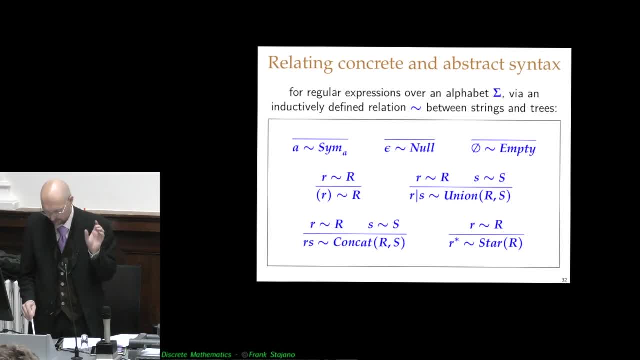 the first part of which matches this regular expression, the second part of which matches this other one, then the whole string matches the combined regular expression, and then this star is something from here you wouldn't see again, but it means, if the string is made of zero, more repetitions of. 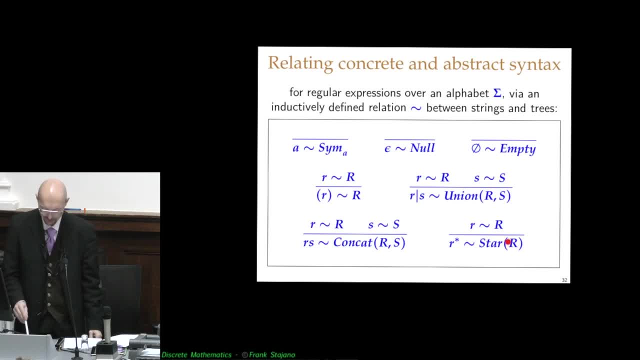 something that matches the original regular expression, then it matches the combined one. and notice here how the brackets in the concrete syntax are completely dropped from here, because the structure of the tree keeps things apart as they should. so I don't need any brackets in here. so the brackets are there. 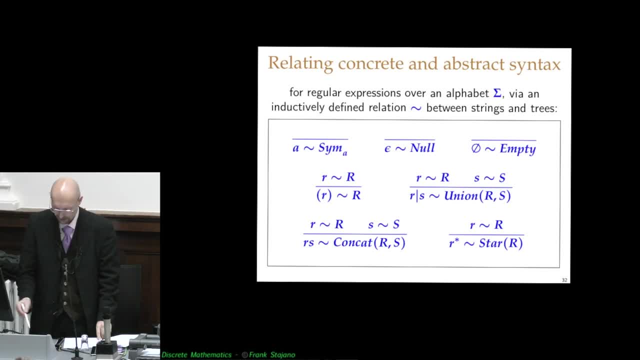 to disambiguate the concrete syntax but are not used, not needed in the abstract syntax.